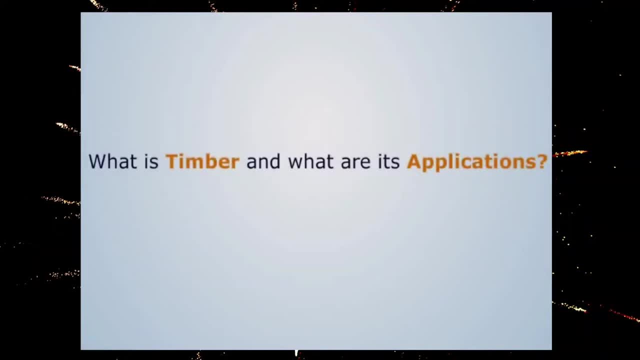 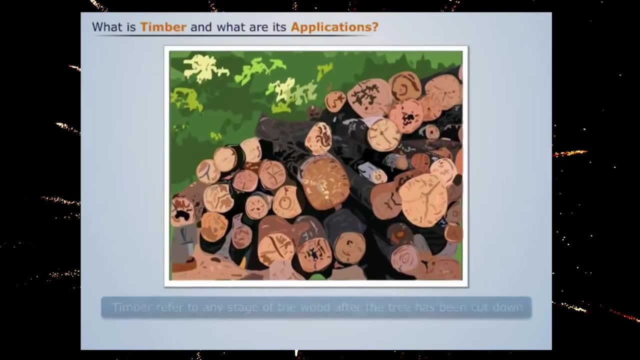 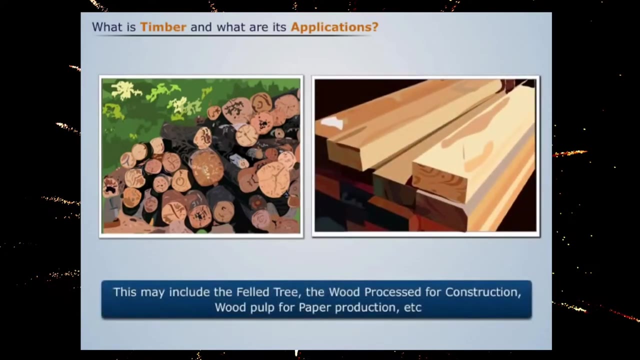 What is timber and what are its applications? Timber is a natural form of wood which is used as a building material. Timber refers to any stage of the wood after the tree has been cut down. This may include the felled tree, the wood processed for construction, wood pulp for paper production, etc. It's 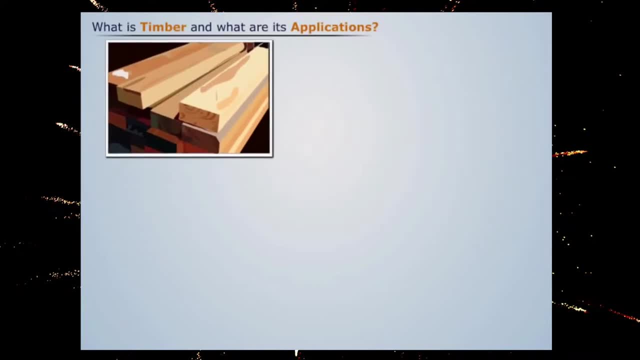 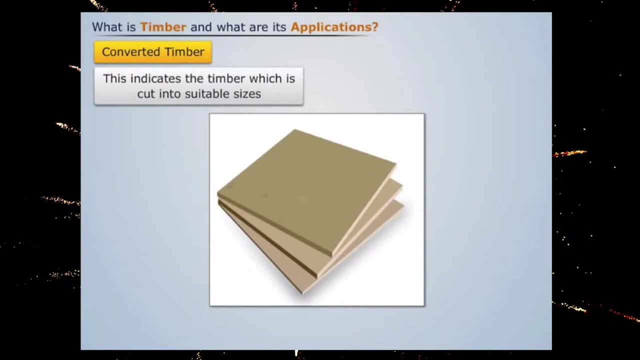 easily available, easy to transport and handle. It is used for building doors, windows, frames, temporary walls, roof trusses, etc. Following terms are used in timber: Converted timber. rough timber. standing timber: converted timber: This indicates the timber which is cut into suitable sizes. Rough timber: this 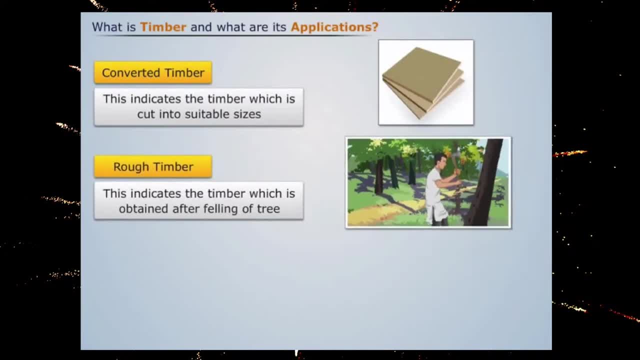 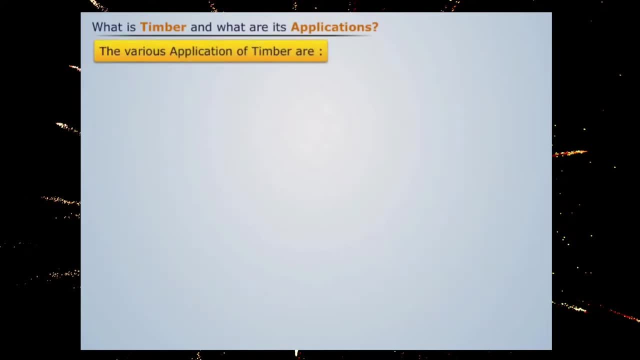 indicates the timber which is obtained after felling of tree Standing timber. this indicates the timber contained in the timber. Timber is used for the construction of a building. Timber is used for the construction of a building Living tree. The various applications of timber are flooring, lining and cladding. 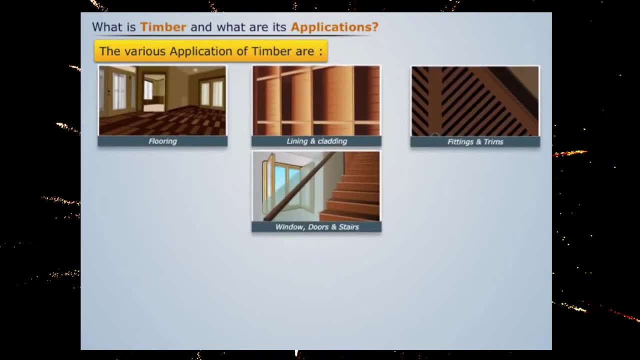 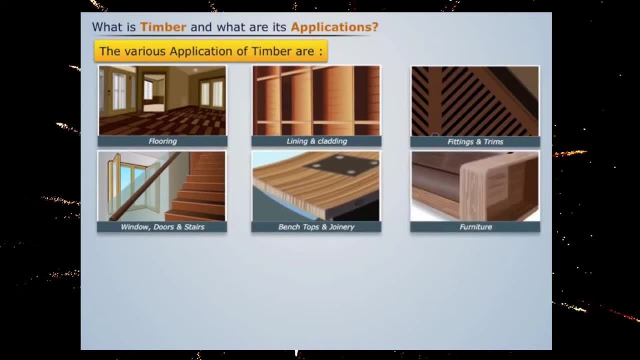 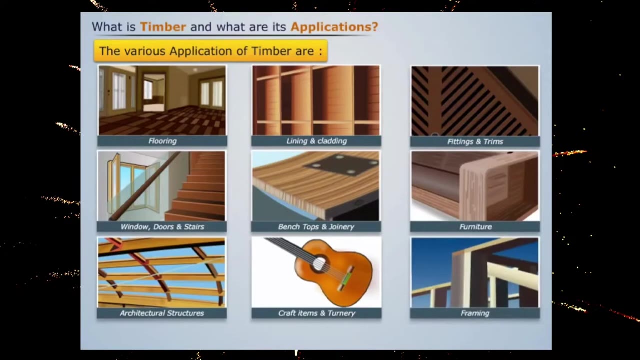 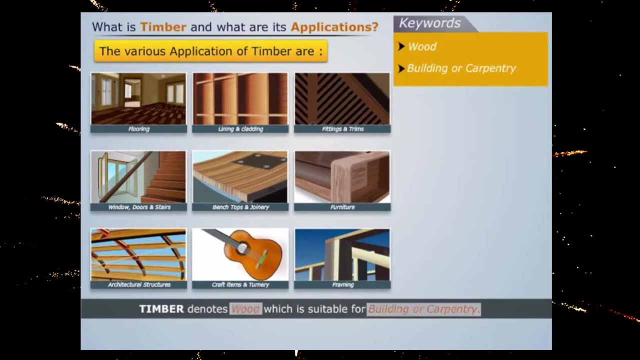 fittings and trims, window doors and stairs, benchtops and joinery, furniture, architectural structures, craft items and ternary framing. Thus, timber denotes wood which is suitable for building or carpentry. The related term is wood which is suitable for building or carpentry. The related term is